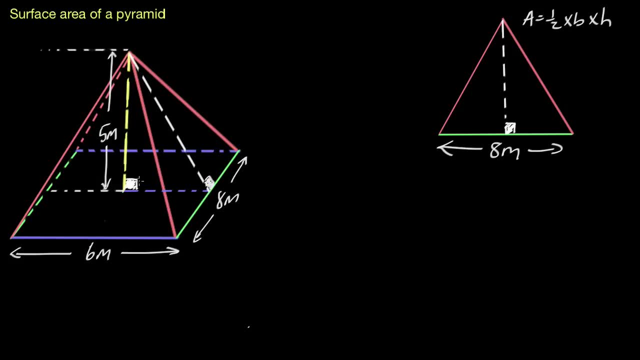 So you need to look back at the pyramid one more time and try to find the length of that dotted blue line. now, if I just put a Little line across here, You can see I'm bisecting 6, I'm cutting 6 in half. 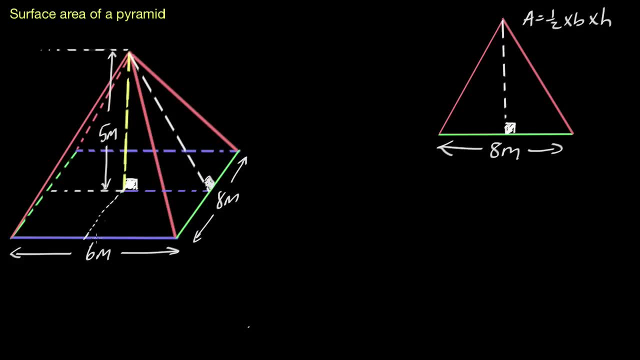 So half of 6 is going to give me 3 meters, and that's the same length as what you've got there in the center of the pyramid, that blue line. So that's where we're going to get our length from. that 3 meters will be right there. 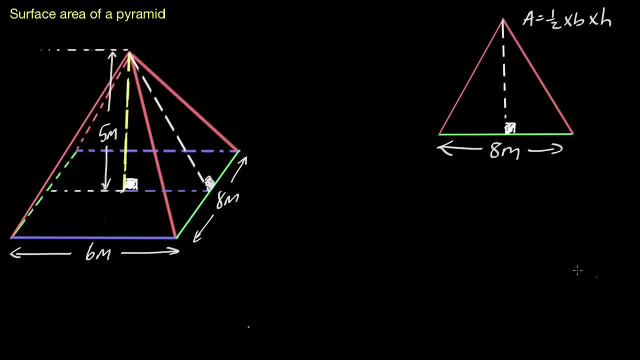 So I'm going to go and take that triangle And I'm going to bring it out so we can work on a little bit and see what it looks like. I'm just going to put it over here And now let's put some values on it So we we know it's 5 meters high. 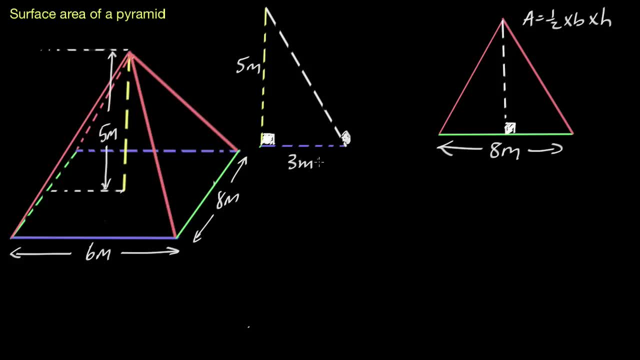 And we just saw that half of 6 is 3 meters. so we now need the value of that hypotenuse. so Pythagoras is a squared plus B squared equals C squared. now C value is the long side, a and B are the two short sides, so 5 squared plus 3 squared. 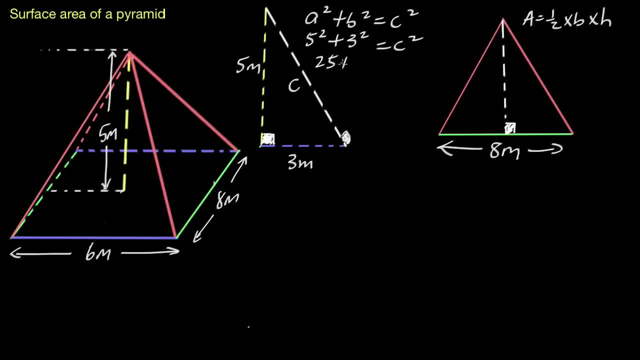 Equals C squared. now, 25 is 5 squared and 3 times 3 will give you 9. So we've got C squared like that. We add these two values together and you're going to get 34. So how do we get C only? 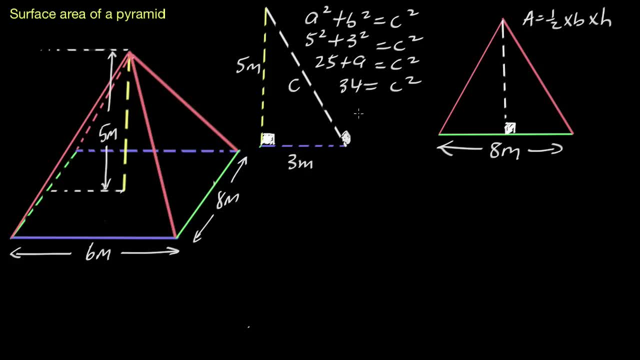 We've got C, squared is 34.. We need to square root it. So C is the square root of 34. now We will leave this answer in exact form like this: if we keep pushing forward and use our calculator, You'll get a number with decimals and that leads to rounding errors. So if we just keep it like that, it's a lot safer. 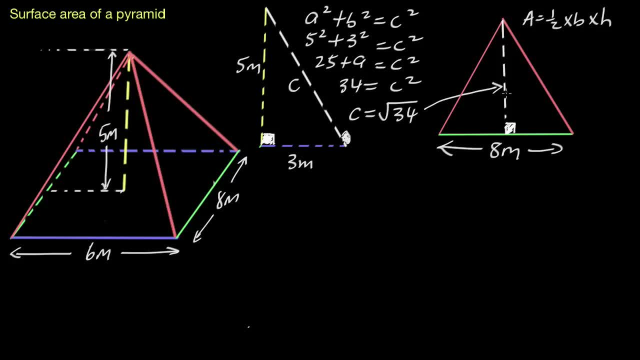 I'm going to say that this height here is the square root of 34. Now, what were we doing with this triangle? We were finding the area of that triangle because we want the area of this face Here on the pyramid. so we now have the base of 8 and we have the height of the square root of 34. 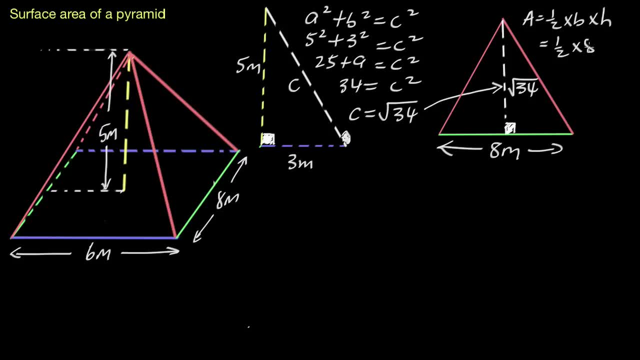 so the area is half times 8 times the square root of 34, and We're going to stop right there because that's enough information. We can use this at the very end to calculate our surface area by simply entering that as it is into our calculator. 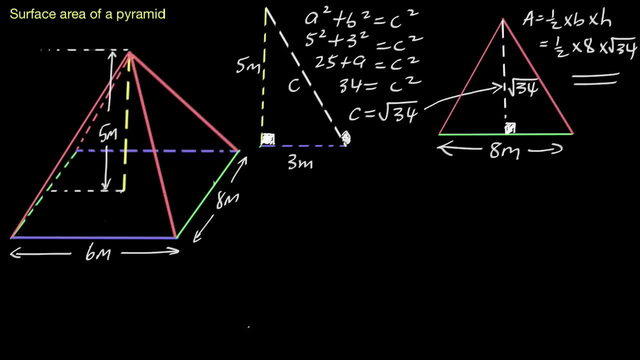 So we'll move on to this front facing triangle. Now that triangle looks like this: you can see, I've got this blue line Which is 6 meters. It's the same blue line down here. So I'm going to say that that's 6 meters and 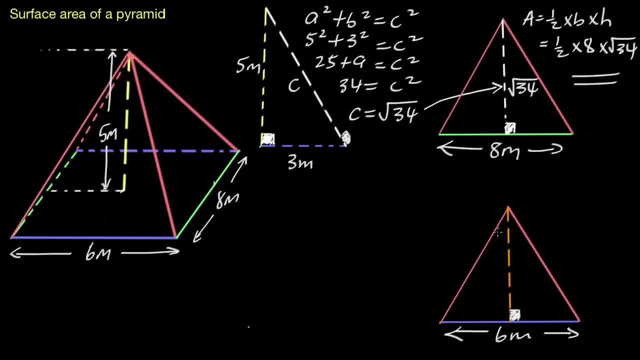 What are we doing with this triangle? Well, same thing we did with the last one: We're finding the area. so the area of a triangle is Half times base, times height. Do we have the base? Yeah, we do. We've got 6 meters, but we don't have the perpendicular height. if you come back to here once again, 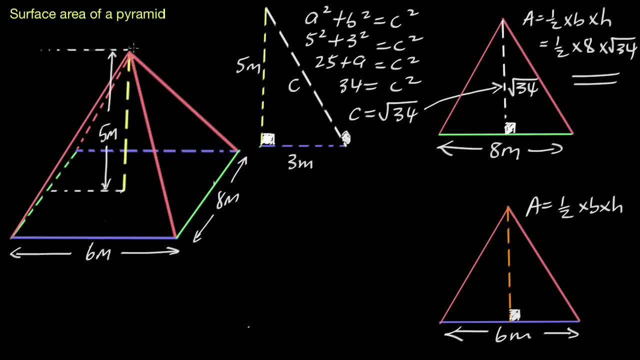 We've got 5 meters, but it's not the same as the slant height that runs straight down that wall there on that angle. so We need to find that, and it's not going to be the same as what we found along this Triangle here, because we've got some different values and you'll see what happens in a second. So here's our next hint. 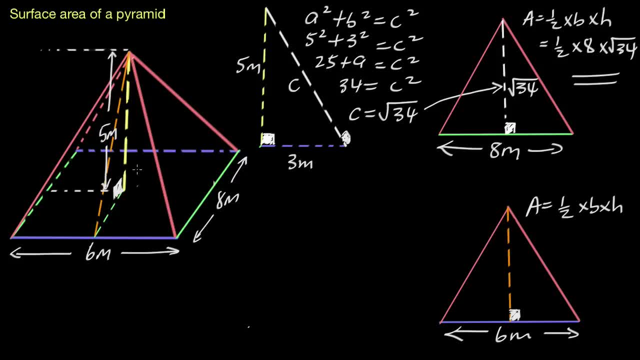 We've got ourselves a triangle inside. It doesn't look like a right angle triangle because it faces towards us, But it is a right angle triangle. It's just the angle that we're looking at it. So I'm going to grab that triangle in a moment. 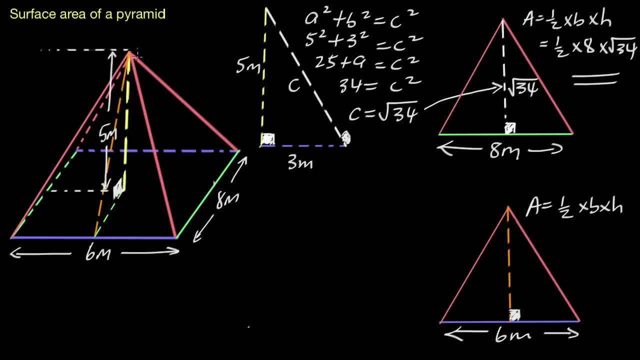 But first of all, let's find out where we get the values from. we know that the height of the triangle is going to be 5, but we need A value for well. I called it B over here. We need the length of the green line. 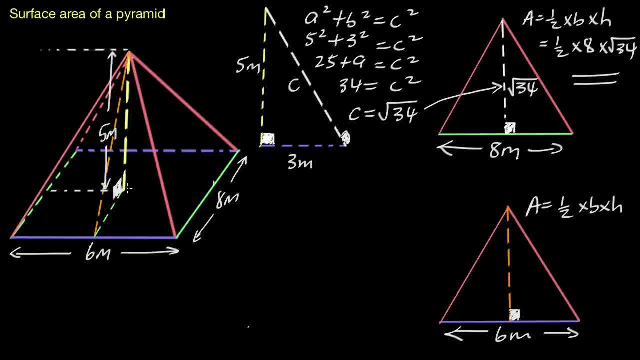 So if you go across from the center of the triangle and instead of bisecting 6 like we did last time, We're going to bisect this way instead. So we're cutting 8 in half. If you cut 8 in half, you're going to find that this green line, the dotted green line, will be 4. 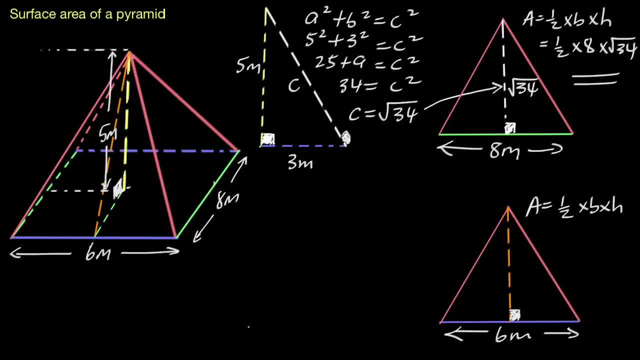 So that's enough information. Now what we can do is pull that triangle out. I'm just going to grab it And we'll move it over to here like that. So let's put our values back on. our height of that triangle is 5 meters, And we saw that half of 8 is the length of the green line, So that's going to be 4 meters there. now, once again, 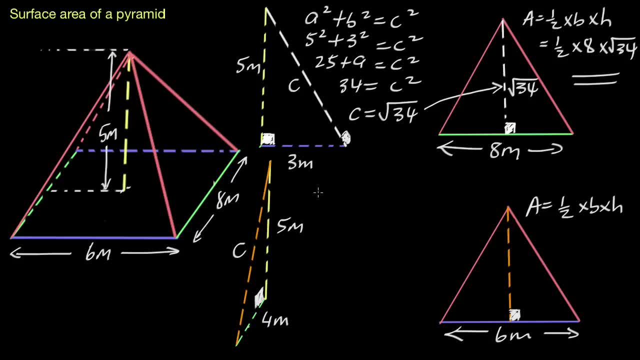 We're using Pythagoras to find a new value of C, So it's going to be: a squared plus B squared Equals C squared. a squared is 5 times 5, so I'll just go straight for the 25 there plus 4 times 4 is 16. 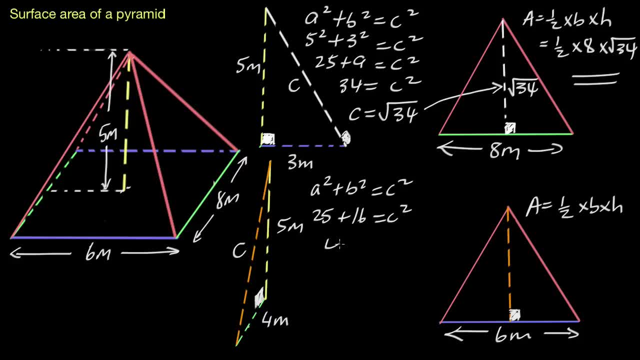 Equals C squared. 25 plus 16 is going to give you 41, So 41 equals C squared. We just want C, though We don't want C squared. So C is the square root of 41 and once again, that is an exact answer. 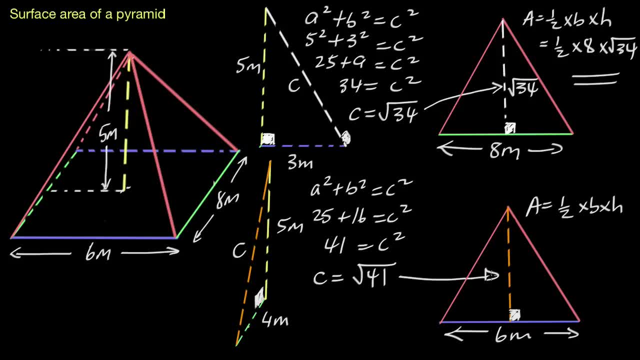 We'll leave it like that. So I'm going to plug 41 into this picture over here. I'm going to say that that height is the square root of 41 because, as you can see, that's an orange line. It's the same orange line that you have here. 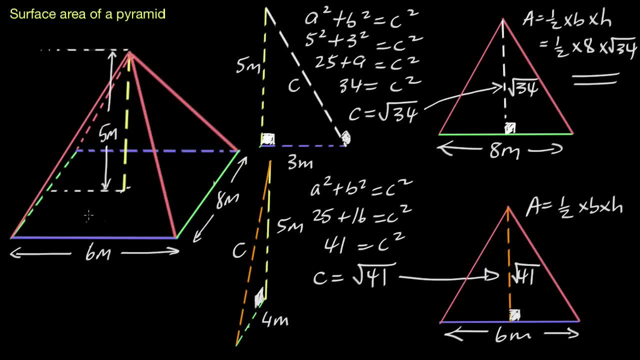 And that's the same orange line that would run down the face of that triangle on that pyramid there. So we are now finding the area of this triangle. So we've got Half times the base. What's our base? 6 meters times the square root of 41, which is our height, and 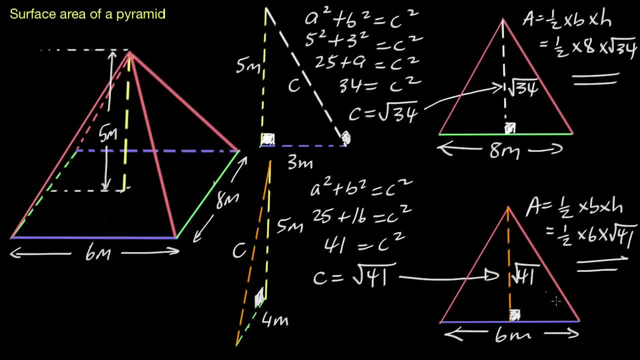 Once again, enough information. We don't need to keep moving forward, because we can use that in one big calculation at the end- And I think we can finish it up now- All we need to do is add all of the different layers together, So a surface area for the entire pyramid is going to be well. we'll start with the base here. 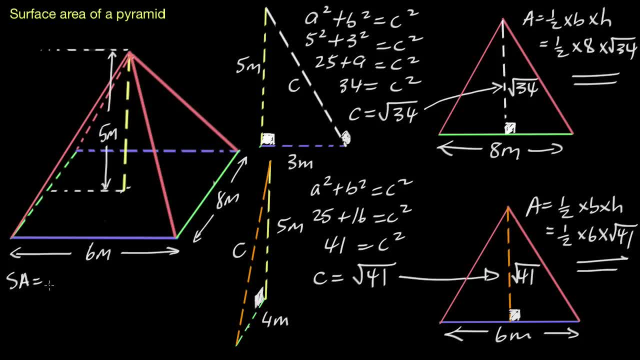 We can see. it's just a rectangle. It's 6 meters times 8 meters, so 6 times 8, Plus we need to start adding on these triangles now. You saw that the right-hand side triangle is this area here, half times, 8 times the square root of 34. 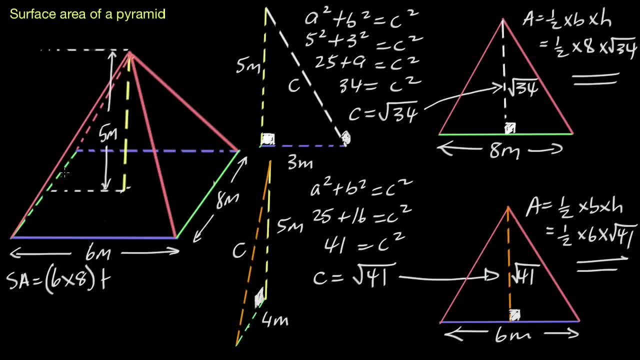 But that triangle has a duplicate on the other side, exactly the same area, So we have two of them. So I'm going to say we need two times, half times 8 times the square root of 34, But we have two more triangles that we need to add, so plus. 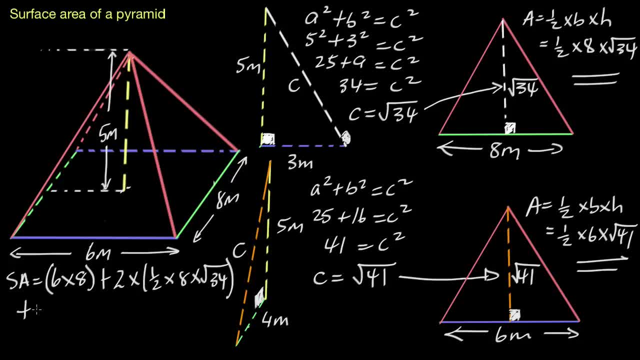 These two triangles, the front and the back one, are both the same size. so two Times, and what are the areas? they're right here, half times, 6 times the square root of 41. Square root of 41. Finally, we just push our equals button, So you do that whole thing in one calculation on the calculator and what you'll get is: 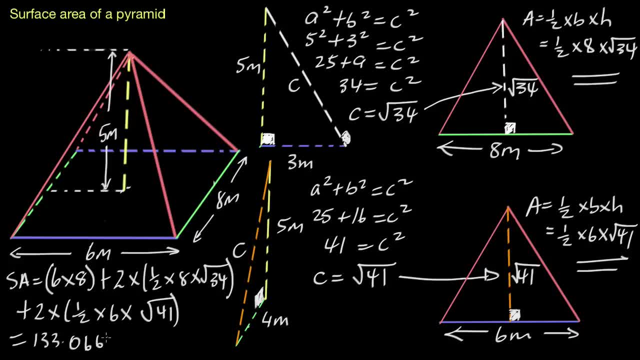 one thirty three point zero, six, six, three, six. those numbers just keep going to round this To two decimal places will give you one thirty three point zero, seven meters Squared, so that there is a total surface area for this pyramid. So that there is a total surface area for this pyramid.